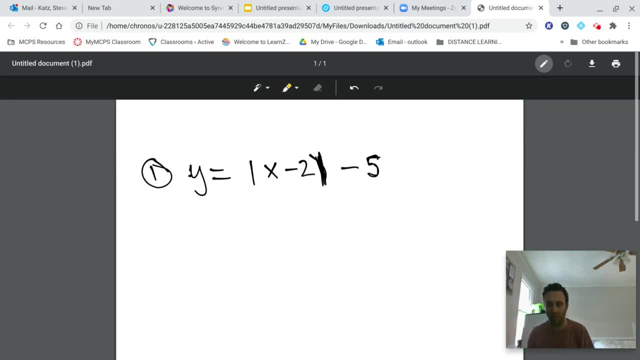 to pause it, practice it, see if you get it right before you get graded on it. So first thing that we're going to cover is absolute value functions. Now remember, absolute value functions are functions that equations that have absolute value embedded in them. So there's. 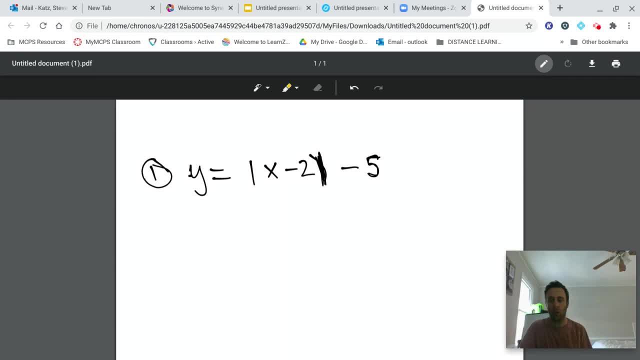 two things you have to be able to do. Number one: you should be able to graph a sketch of this without actually putting anything into the calculator or finding any points. So that's the first thing we're going to talk about. So, if you want, you can pause the video. 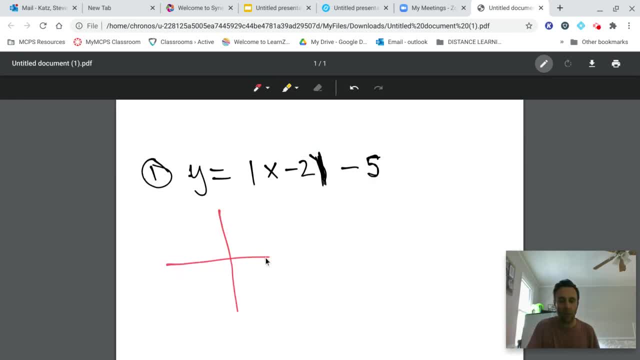 and try to just do a rough sketch of this And hopefully, if you got a chance to try this on your own. you said that these two numbers actually tell you where the vertex is. Remember the vertex of an absolute value equation is where the two lines or the rays meet And here, inside the absolute value. 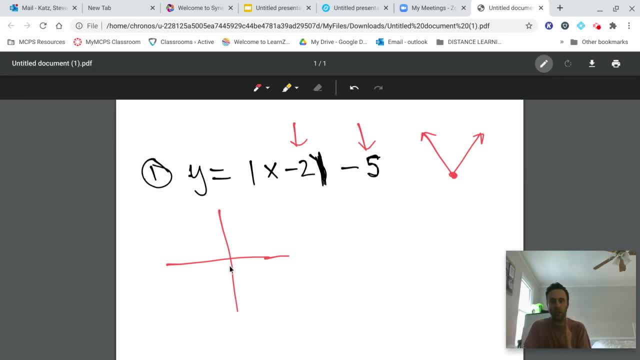 it's going to shift it or transform it left or right. So the vertex is going to go from zero, zero and this negative two is always the opposite. So if it says negative two, it means the vertex shifts to the right two, And then this negative five tells you up, or 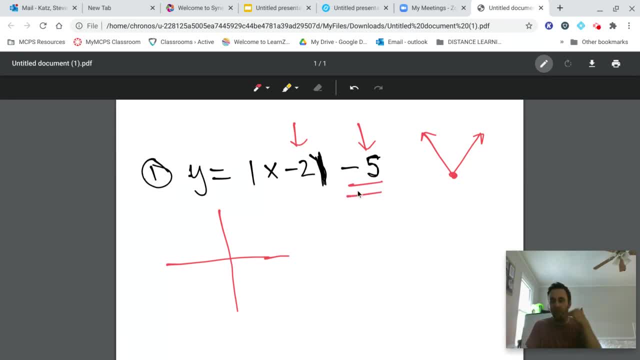 down. But if it says negative five, it means down, If it says positive five, it would mean up. So your vertex shifts over to the right two and then down five. So your vertex is at the point two negative five. And that's important to know. Now, absolute value functions. look. 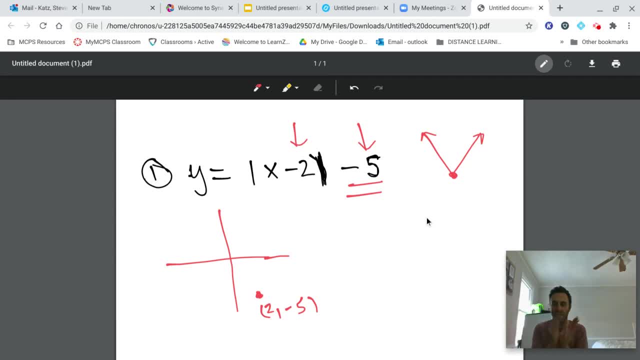 like a V. They kind of represent any kind of a V shape. So people always ask: well, how do I know how wide to draw If you're just sketching? not that important to really know exactly how wide to make it. But one thing that I 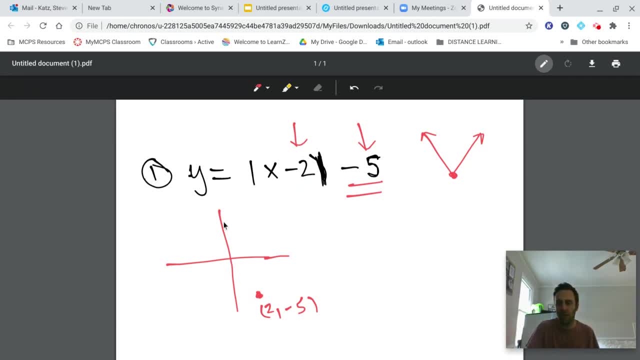 do tell my students is that you kind of want to know where the Y intercept or the vertical intercept is, So where the V or the absolute value function is going to hit this line, X is going to be zero. So the easiest thing to do is just plug a zero in for X and solve. 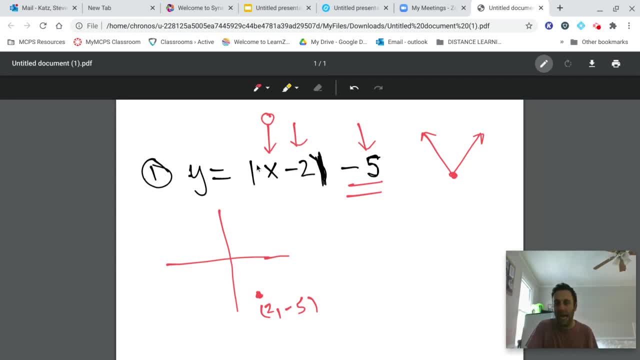 it. So zero minus two is negative two. The absolute value of negative two is two positive two, And then two minus five is negative three. So that means at zero negative three. it's going to hit the Y axis And it kind of gives you a little bit of a, you know at least. 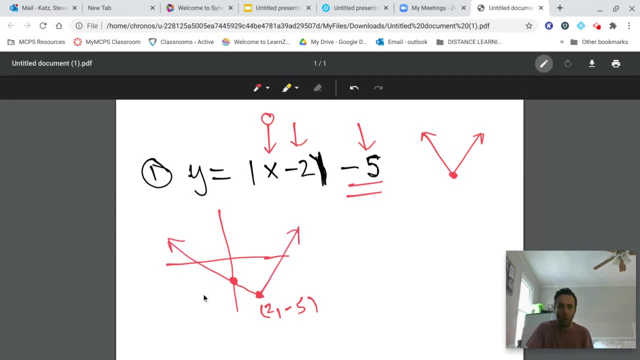 a little bit of a shape that you could kind of follow And if you want, you could always mark that point. The Y intercept is zero negative three, And again we got that from putting the zero in there. So the other thing you have to be able to do is kind of what we just did- is, if I asked, 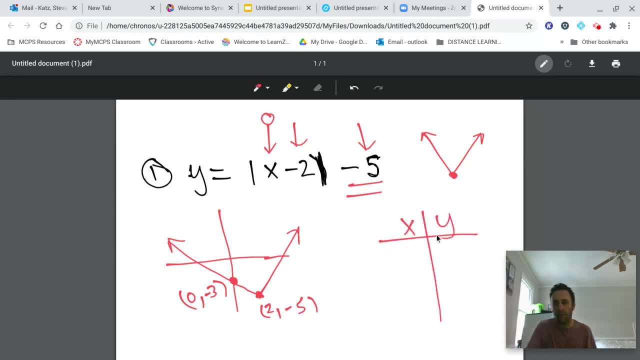 you to find some values that work for this function, now that you know that the vertex is two. so I'm going to put the two like kind of in the middle And then I'm going to put the zero in there. So I know that if I go greater than two, that's going to be the 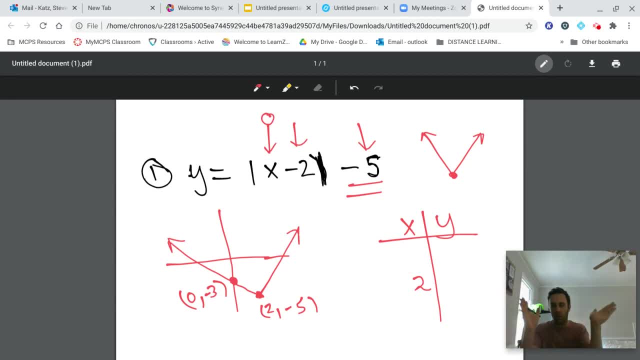 point that the function is going to go higher or lower depending on where I am. So I'm going to go from two is the point of my vertex. I'll go from zero, one and two, and then I'll go two past it, I'll go three and four And then just being able, you're ability to just. 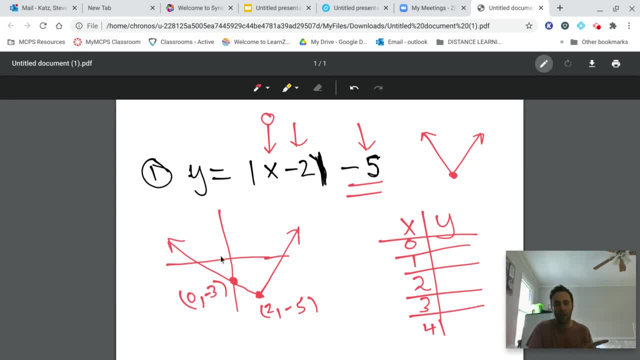 write in the points is also important. So if I plug in a zero, we already know what we're going to get. We're going to get out a negative three, because I've already done that. If I plug in a one, one minus two is negative. 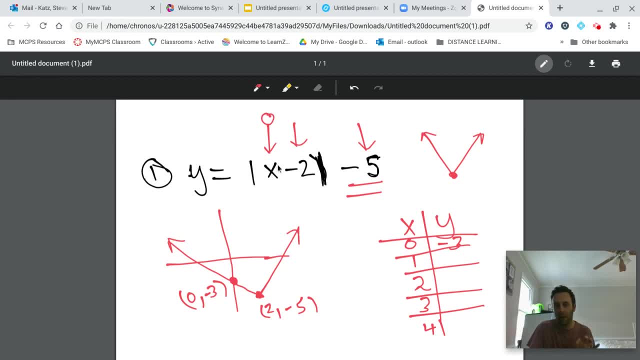 zero, 1.. Negative 1 minus 5 is sorry. 1 minus 2 is negative 1.. The absolute value of negative 1 is 1.. And 1 minus 5 is negative 4.. What else we got? 2.. 2 minus 2 is 0.. Absolute value of 0 is 0. 0. 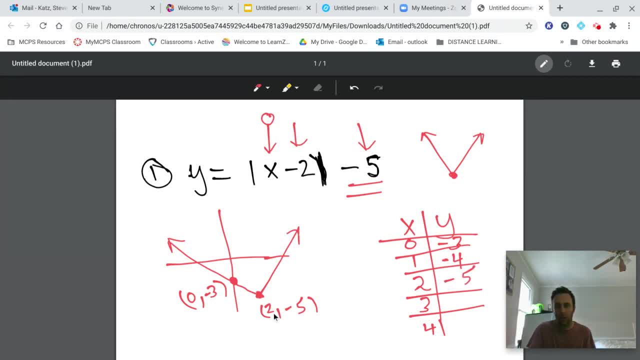 minus 5 is negative 5. 3. We already actually we knew that point because that was the vertex of 3.. If I put 3 minus 2, now I get positive 1. But absolute value of positive 1 is still 1.. 1 minus. 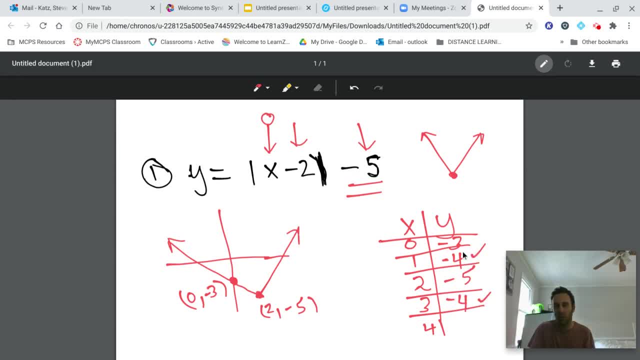 5 is negative 4. And you're going to see that they're going to start repeating. So this point, I know, is going to end up being negative 3.. But just to double check, 4 minus 2 is 2.. Absolute. 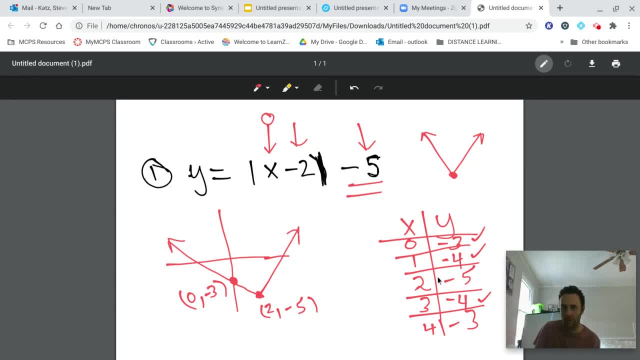 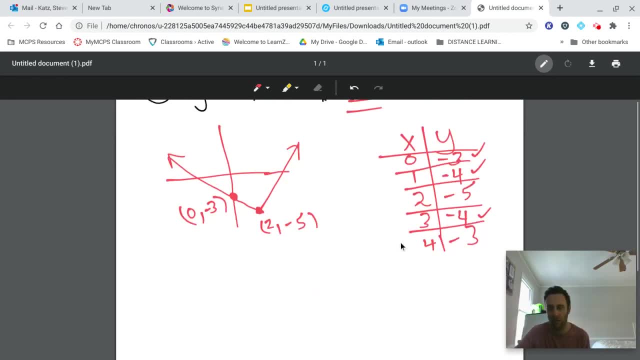 value of 2 is 2.. 2 minus 5 is negative 3.. And then that's how you get some points in absolute value. Okay, So right now I'm going to say: you know, obviously go back and repeat that I'm going to. 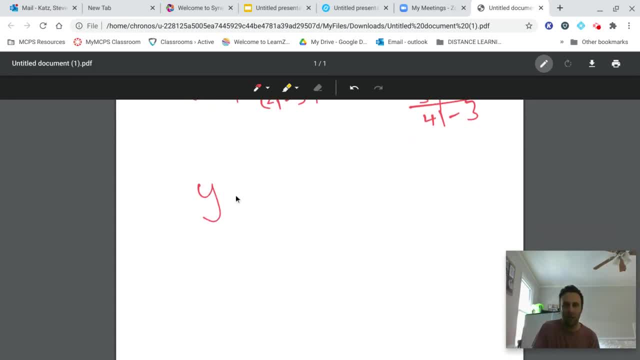 give you a couple different questions about. the absolute value of y equals the absolute value of x plus 3. Minus 4.. Okay, So the questions that we did ask you remember? you saw if they're right or wrong. but we asked you about where the vertex would be. What would be the y, the coordinate of the y? 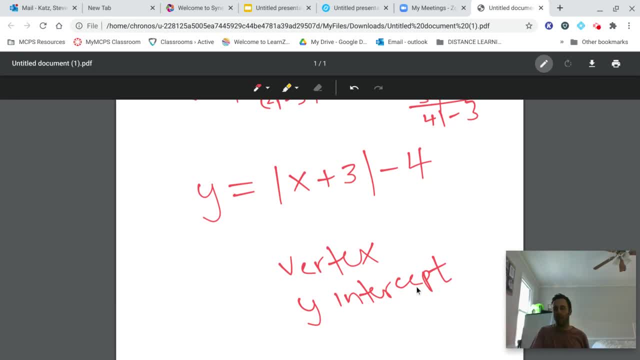 intercept And also, and remember, these are all things that we did in back in the video above. And then last, what would y equal if x was 10?? Okay, And then obviously, if you plug the 10 in it's 13. Absolute value of 13 is 13.. 13 minus 4 is 9.. So the point on our function would be 10 comma 9.. 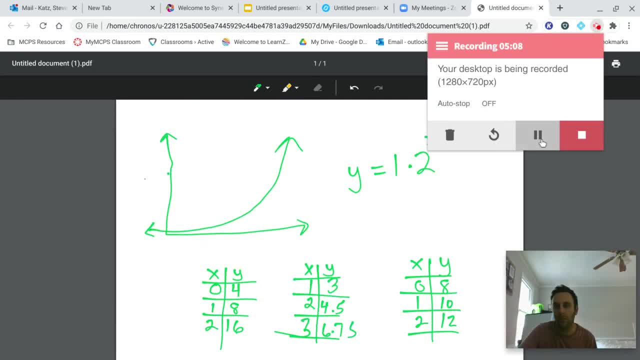 Okay, So All right. So the next kind of problem we went through in class is we did a different type of function. We switched from absolute value functions to exponential functions, And this is called exponential growth. A couple things that I want to remind you of before we go into some. 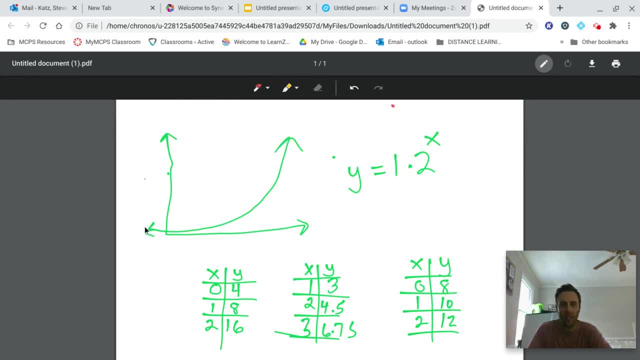 questions that we did in class. So we did a different type of function. We switched from exponential growth. A couple things that I want to remind you of before we go into some questions that we did in class is number one: exponential growth. It looks like it's like this is completely flat. 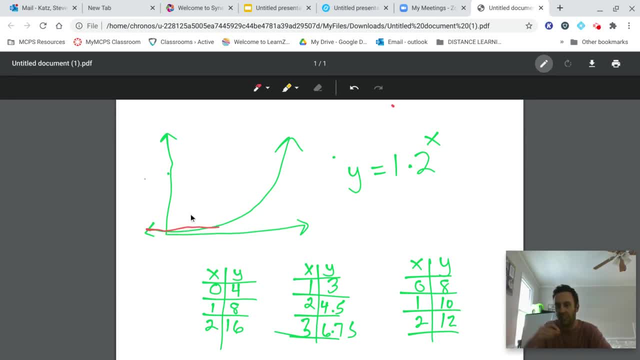 It's not. Even though it looks flat in an exponential function, it's still increasing. It's just increasing at a very small amount And as you get later in the function it's going to just kind of shoot up like this because you're now multiplying by bigger, bigger numbers And it's 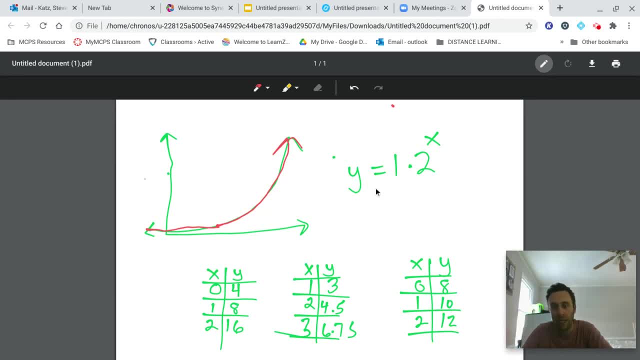 going to get a lot faster, a lot quicker. Now, this would be an example of the equation. that's an exponential function. We know it's exponential because it's to the x power. This number right here, remember, is your growth factor. That means that you're multiplying this by 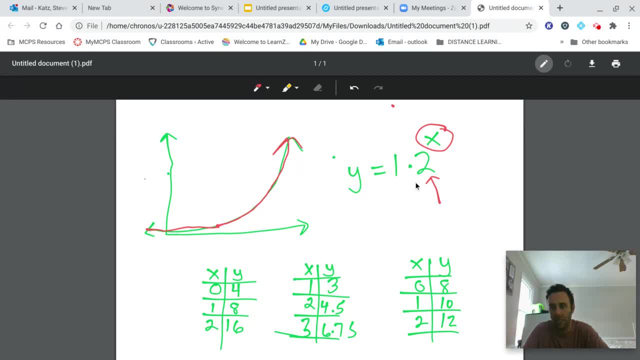 two. So if this graph is times two times two times two, it would be two to the x power. The times one in front is actually the y intercept. This means that the graph crosses the y axis at zero one. It's the starting point. So before this started growing, you were at zero one Before day. 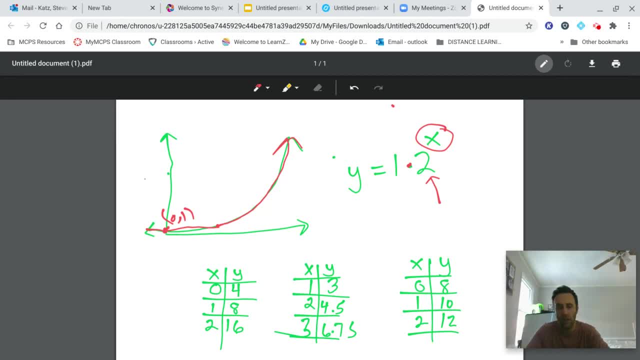 one at day zero. you were at one and then just kept growing. This would be an example of like bacteria. If you had one bacteria and it doubled every minute, this would be an example of why bacteria grow so fast: because eventually you're going to start. 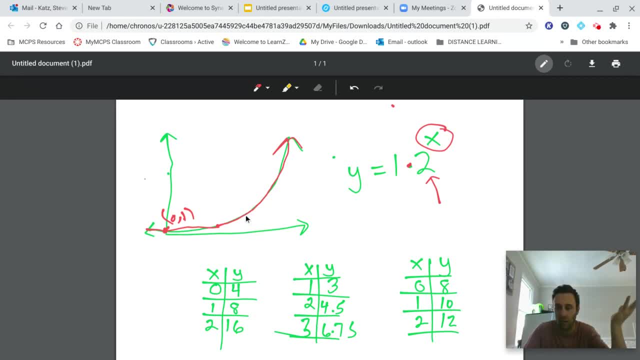 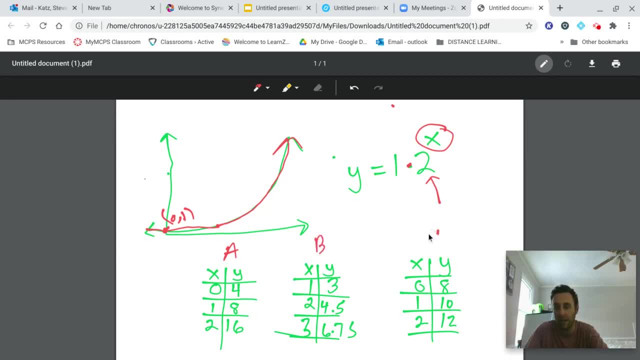 So, first thing, you could kind of answer this out loud or pause the video. But which one of these functions are exponential functions? So hopefully you said A and B, because A and B, if you look at the y's, the y's are being multiplied by something every time In letter C. let's do this one first. 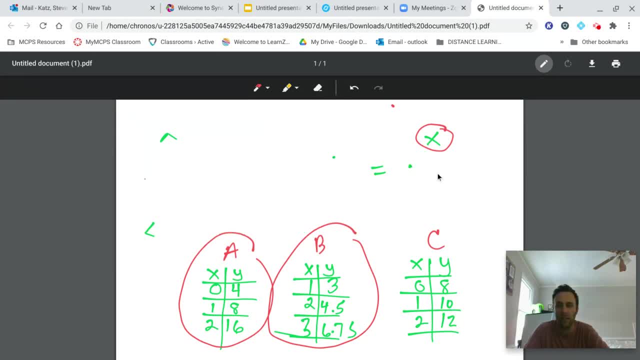 I'm going to erase this, so I get rid of this. so I could write on the top of it. So if you have a function where it gets added or subtracted every time, So in this one you can see it goes plus two, plus two and plus two. In that case- remember that's a linear function, So we write. 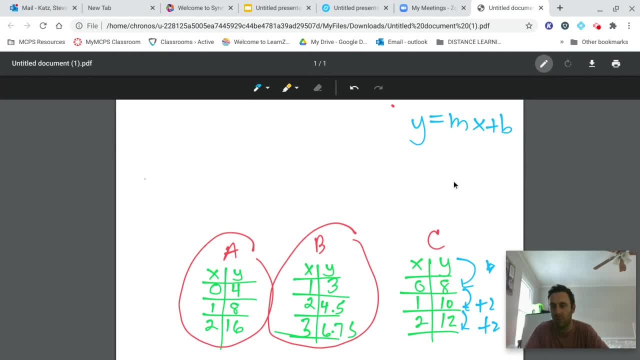 linear functions. One way that we learned in, I guess, back in September, October, is: y equals mx plus b. The m, the slope, is actually what's happening to the y as x increases by one. Well, you can see, it's going. 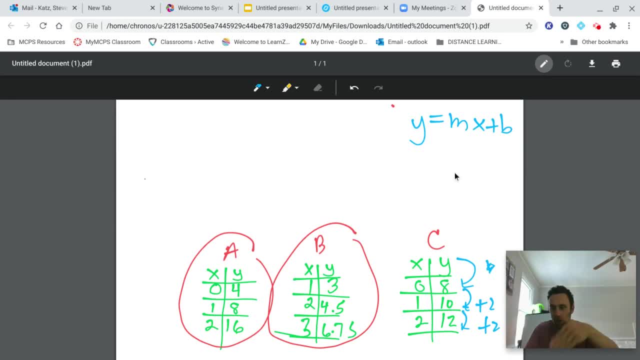 two. It's getting times two every time. Plus two plus two, plus two actually means you're multiplying the x times two. So when we go to write this, we put the two or the number you're adding in front, right in front of the x, and that's the slope, And then the b is still the. 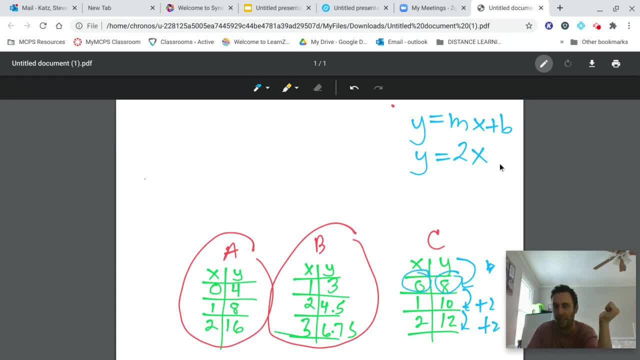 same, It's the y intercept. When x is zero, what's y? And in this case it starts out at 808.. And this would be the example of a linear function and how to write it. But what we did in class. 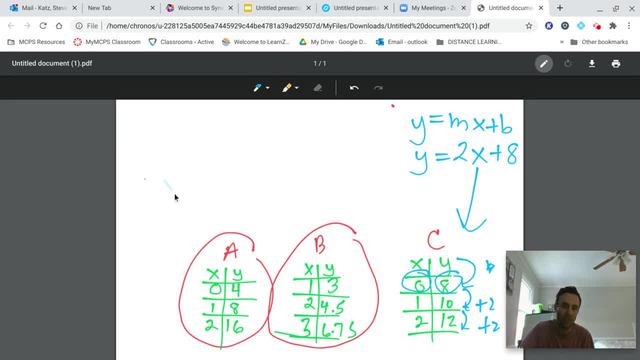 sorry, we learned to write exponential functions. So how do you write an exponential function for this? Well, the format is always: y equals b times a to the x power, okay- Whereas a is the growth factor- We just talked about this- And b is the y intercept. So in this problem, the y intercept is: 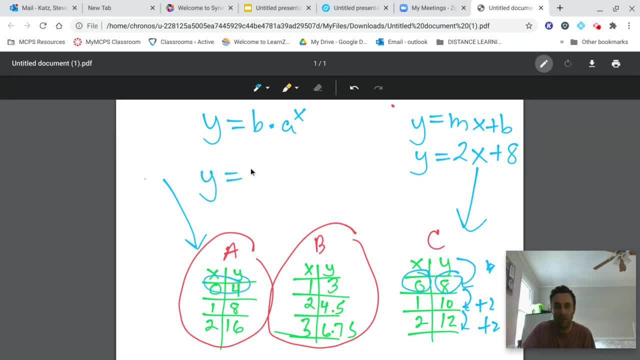 four. So y equals, or f of x equals four times. And then what is the growth? What's being done? It's being multiplied by two. We just don't know how many times we're multiplying by two. So that's two to the x power, Because two to any 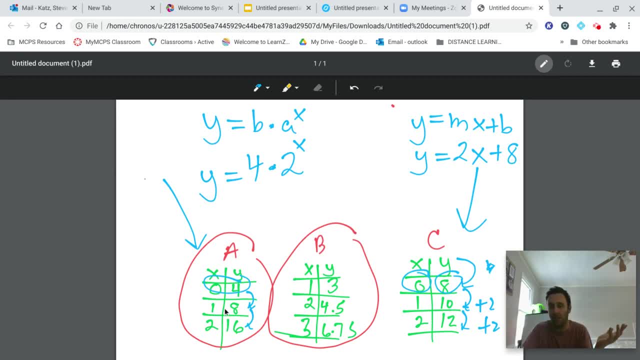 just means you're multiplying by two. You just don't know how many times. Maybe you do it one time, Maybe you do it two times, But either way, this would be the exponential function for a, And go ahead and try exponential function for b While I erase this. you could, of course, 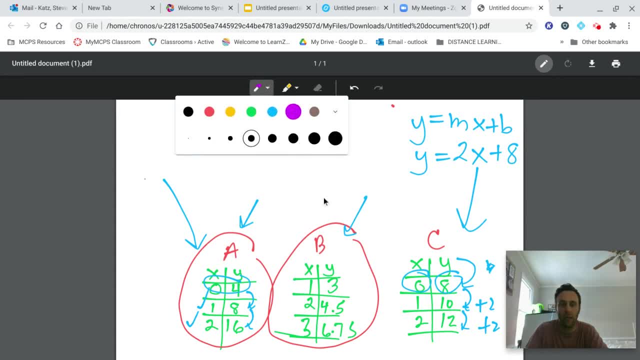 pause the video and see what you get. So for letter b or function b, I guess. well, it doesn't have a y intercept because there's no x of zero. So the first thing I want to do is: well, first of all, 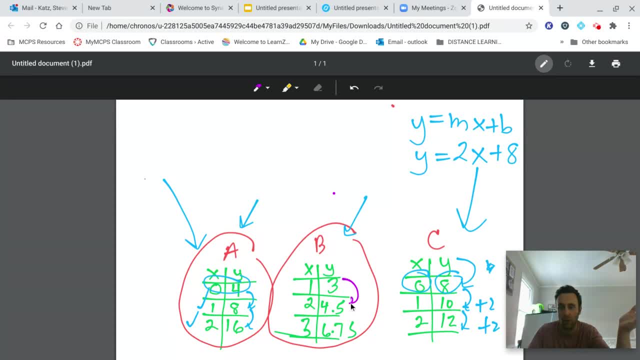 is a y, It is a exponential function, And if you do three divided by 4.5, it's actually 1.5.. You're actually multiplying each of these by 1.5.. And I know that because if you do this, divided by this, 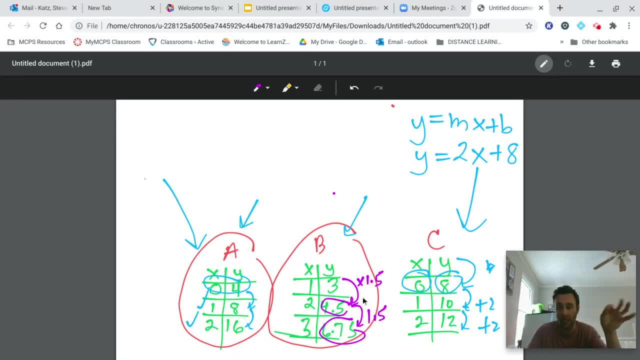 the number before it, you keep getting 1.5.. So three times 1.5 is four and a half. Four and a half times one and a half is 6.75.. So I can see that you're multiplying by one and a half every. 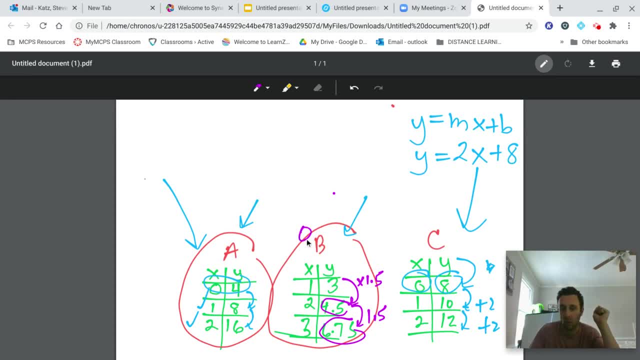 time. Now all I have to do is figure out what's the. when x is zero, what's y? Well, I just have to bring it back one time. So when x is zero, what's y? Well, I just have to bring it back one. 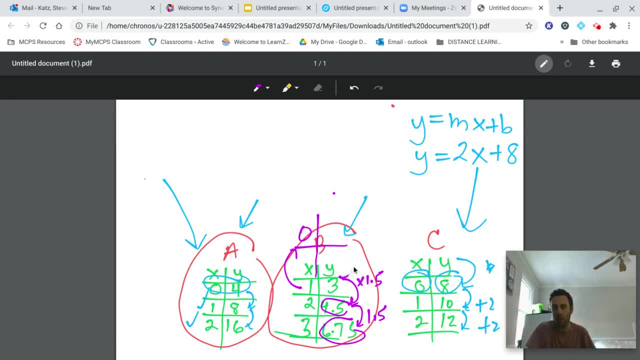 time. So, when x is zero, what's y? Well, I just have to bring it back one time. So, when x is zero, instead of multiplying by 1.5, I'm going to go backwards. I'm going to divide by one and a half. 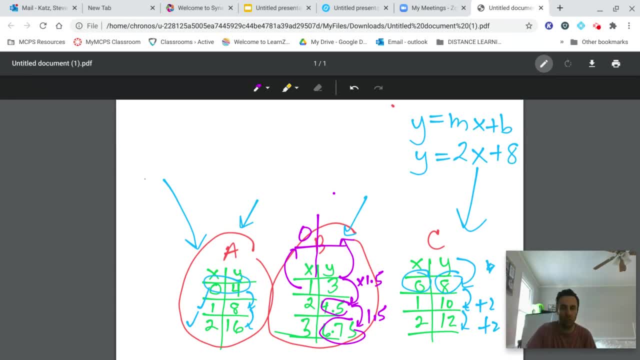 So three divided by one and a half is two. So I know that a point on my function is zero too. So to write this function, y equals or f of x equals the y intercept two times the growth factor to the x power, And this will get you any. if I plug in an x, you're going to get the y. 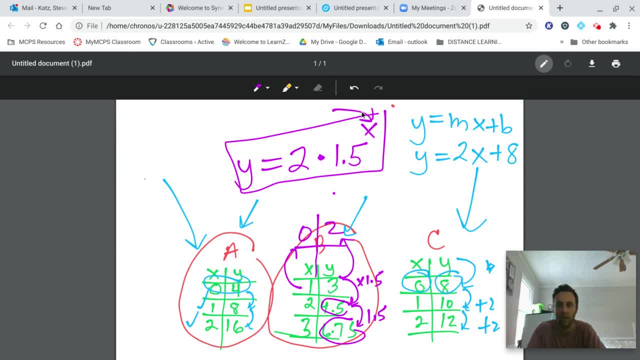 for this particular function, Like if I plug in a three, 1.5 to the third- this is this spot right here- is 1.5 times one and a half, times one and a half, And then, if I do that times two, I promise you you will get 6.75 or six and 75 hundredths. Now let's try a couple for you. 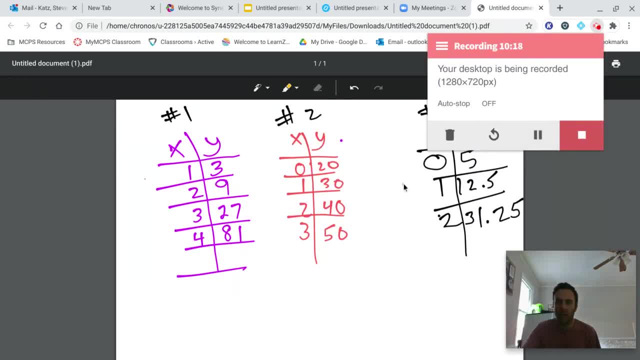 All right. So basically, here are three problems that the first question I'm going to ask you is which one of these are exponential functions or exponential growth? Which one of these are growing exponentially? So hopefully you picked number one, and number three are actually being a growing exponentially. 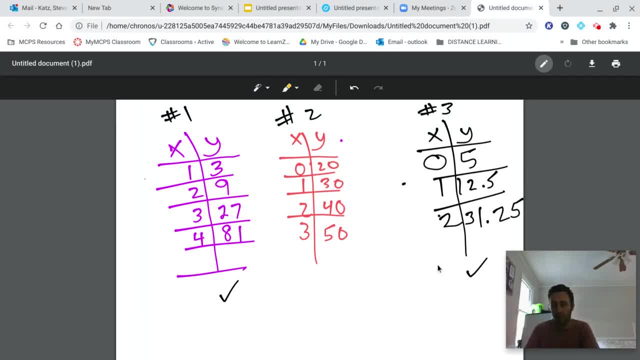 Okay, So those are the ones that you're going to make sure you have exponential functions for. So the first thing is go ahead and what is the equation for the linear function number two, and make sure you go back and figure out if you're, if you forget how to do that. 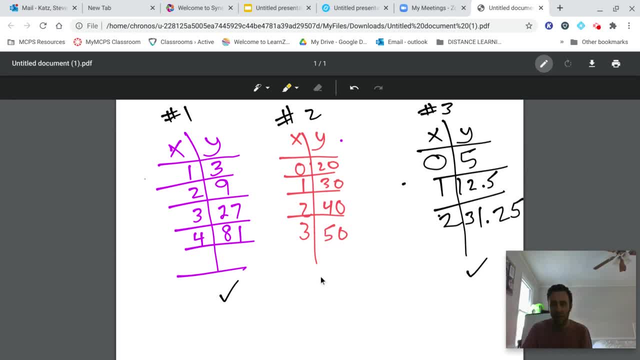 just go back in the video and I do an example of that. So here what's happening is it's going plus 10, plus 10,, plus 10.. So it's y equals 10x and the y intercept is 20.. So it's plus 20.. And that's the equation for that one. So go ahead. 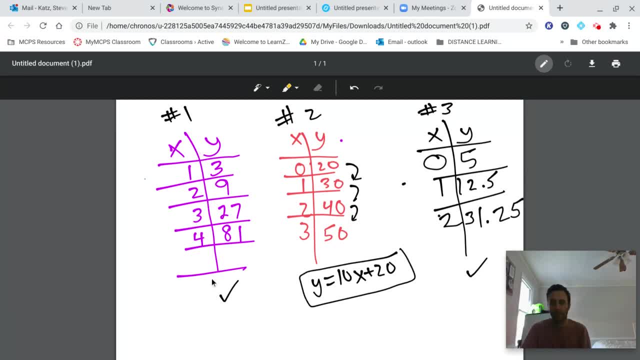 right now and find the equation for the purple. Now again, this is exponential, So hopefully you said so. first of all, there is no y intercept. Oh, so you had to go back to zero, get x to zero And instead of multiplying by three, if you want to go backwards, you would divide by three. 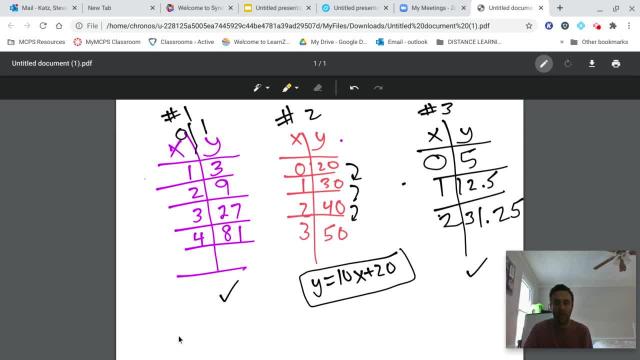 Now, one thing I do want to tell you is that there are some times there are actually two ways to write this. So the way that we let you write this, or one of the options, was one times, because the y intercept is one. 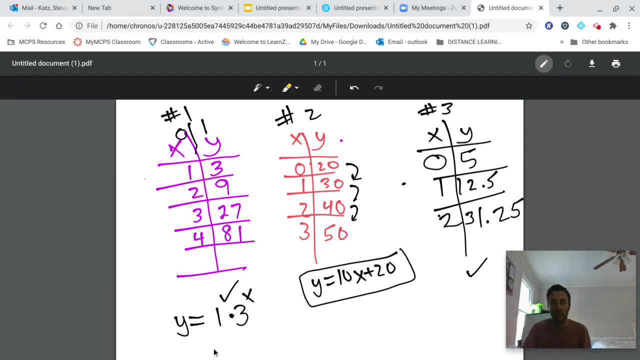 and it's the growth factors three to the x power. You might also see this as y equals. in other cases You might also see this as y to the three x power, because if you don't see a number in the front, it means it's times one, It's not times zero, because you have to multiply And if you 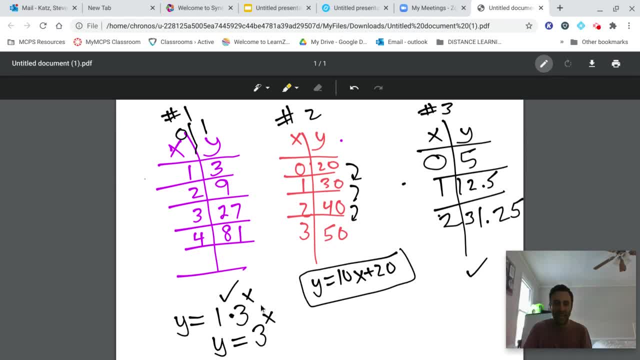 do zero times anything, you would just get zero. So if you ever see an exponential function with just like the something to the x power, you assume that the y intercept is one And we'll talk more about that. but just I wanted to. it was worth noting, right. 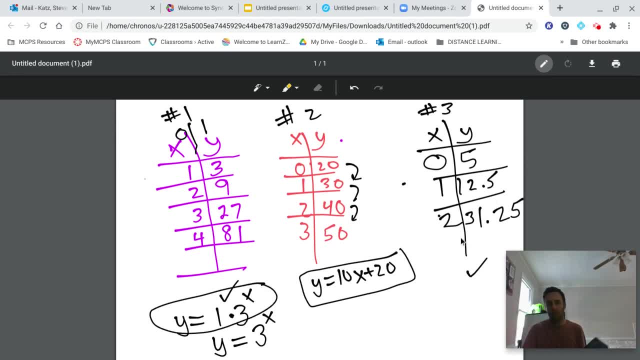 now. And now can you figure out the equation for this one? So first thing I did is I had to figure out what are we multiplying by. I mean, we already told you so that it was a multiplication problem. So in order to figure out what you're multiplying by, I just divide these two numbers, 31 and a.